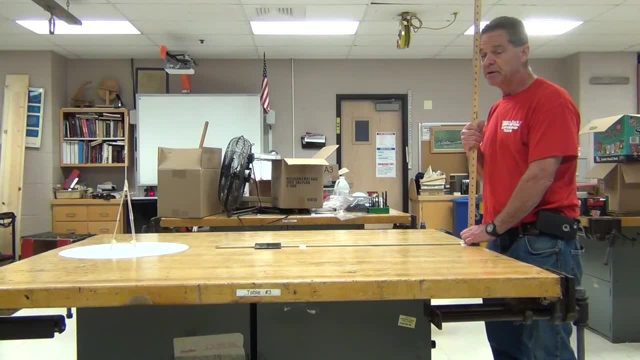 I'm lining up my line of sight, my eyesight also, at the edge of the table, right My body's right here and I'm keeping my eye in just the right spot. that's directly, you know, straight up from the edge of the table. 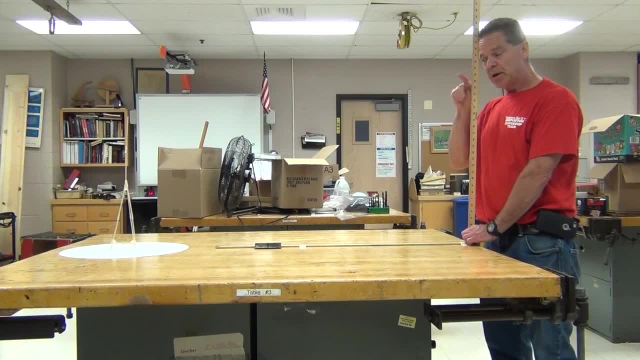 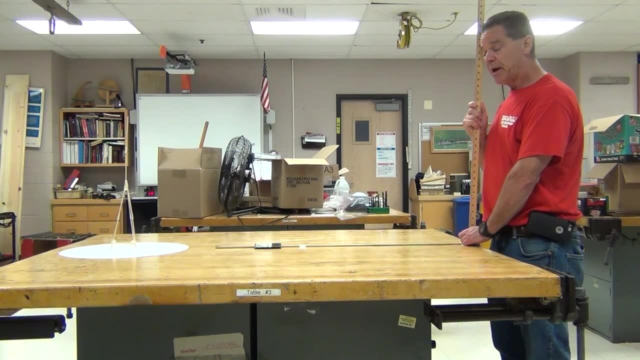 So I've got a right triangle right here and I'm looking down at the mirror glass right And I can see the top of that tower touching the magic marker line on the mirror. And if I couldn't, I'd either need to move the mirror back and forth. 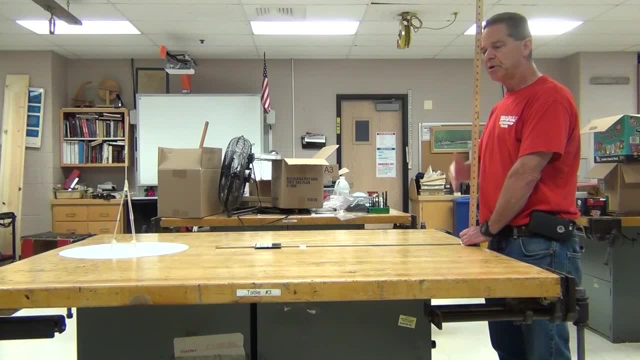 If I've got my eye positioned in just the right spot, so it's a certain height, I can go here and look and see that it is, I would say, 74 centimeters from the top of the table, 74 centimeters from the top of the table to where my eye is. 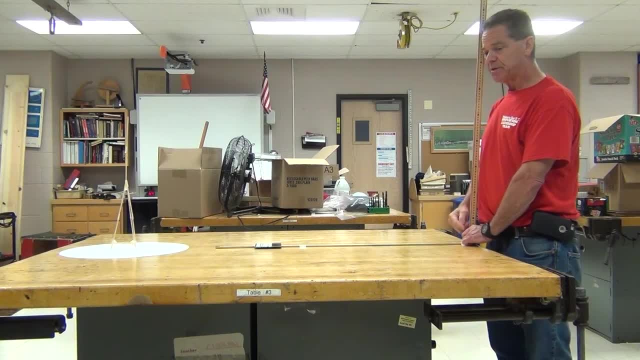 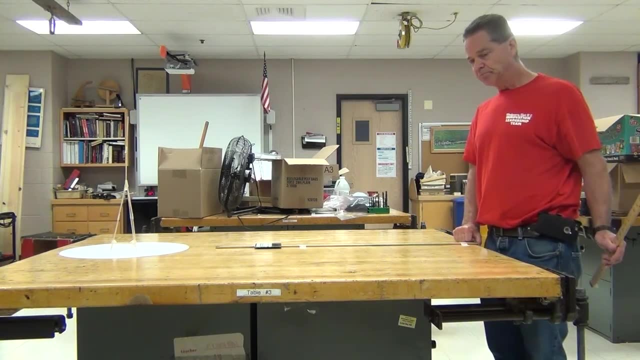 The center of my eye. okay, And then. so that makes this height over here 74 centimeters. The distance would be this distance here to the center of the mirror, which is somewhere around. I'll have, I'm not going to do. 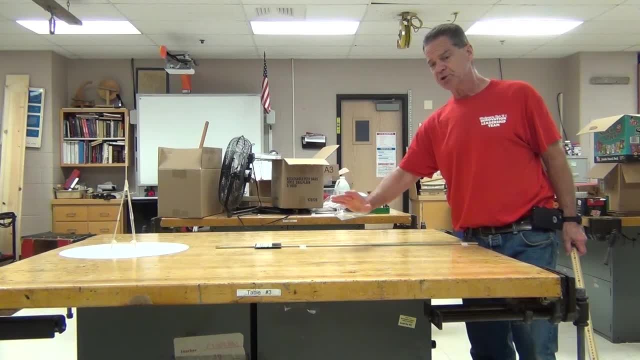 See, I'm not going to do the numbers for you this time. I'm just going to explain it and show you. You'll have to figure it out on your own when you do it, But the center of the mirror is somewhere around 80 centimeters. 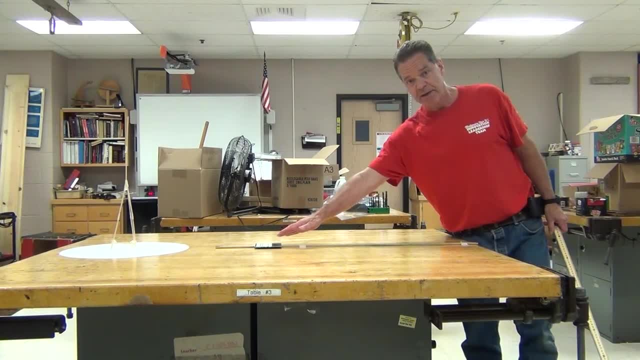 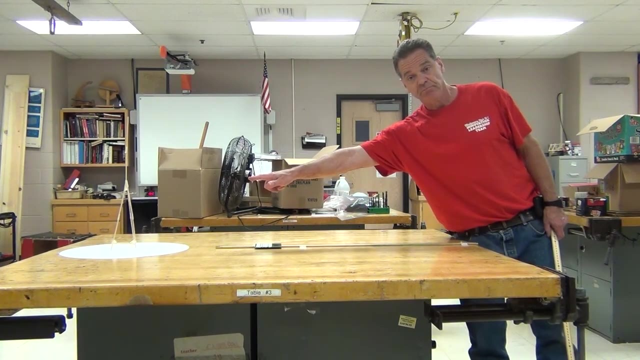 So from the edge of the table to the center of the mirror to that line on the mirror is 80 centimeters right. That also means that that line is, say, 43 centimeters from the point underneath the tower right. 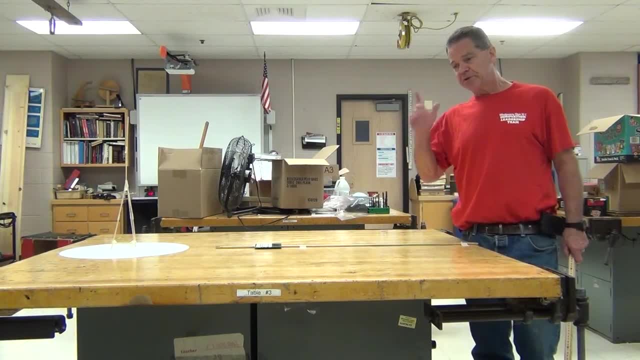 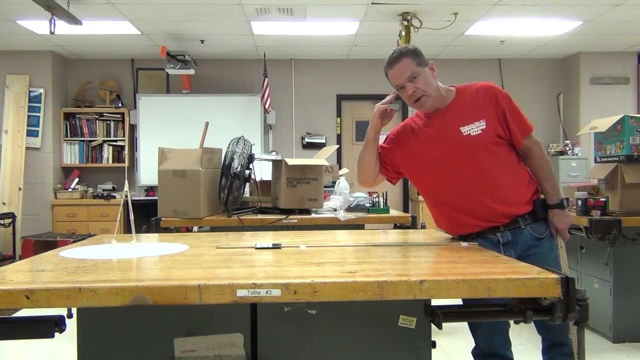 So, basically, what we've done. Well, here's the other thing that's important to know. Mirrors have an interesting feature. If I'm looking down here and my line of sight, these light rays are coming in at a certain angle. they reflect off at the exact same angle. 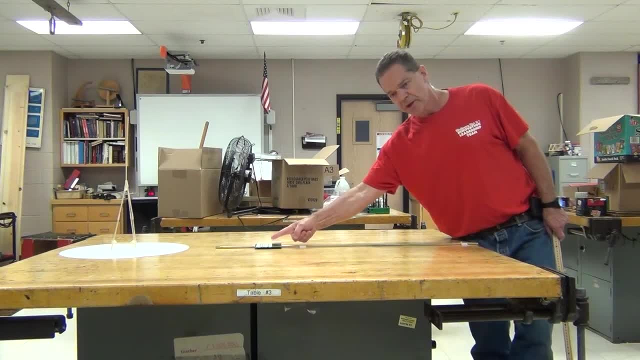 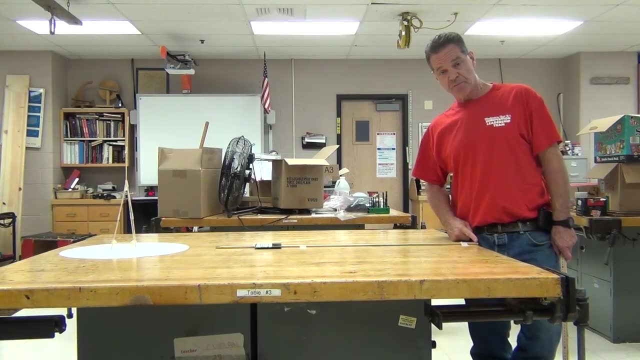 So I've got two triangles that have this angle right here, the same. I've also got those same two triangles with a 90-degree angle, the same, out here. So I've got two similar triangles right, And if I can figure out a ratio between my height and this distance, 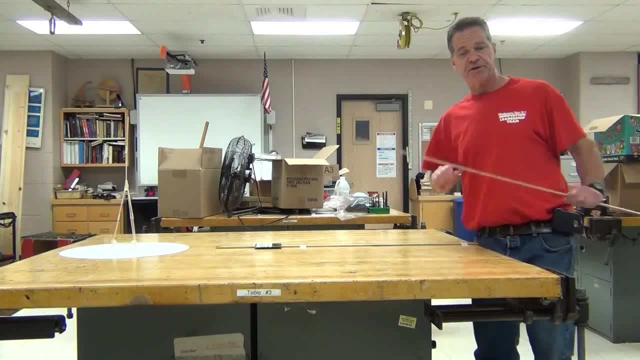 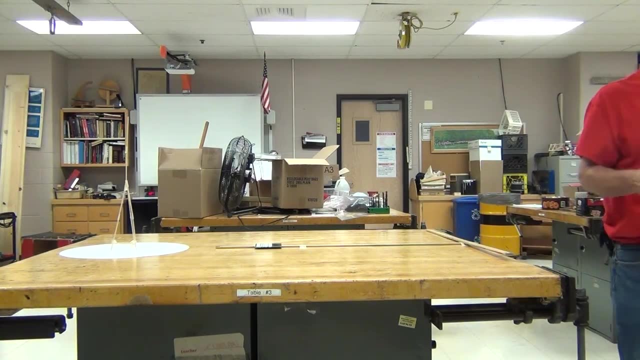 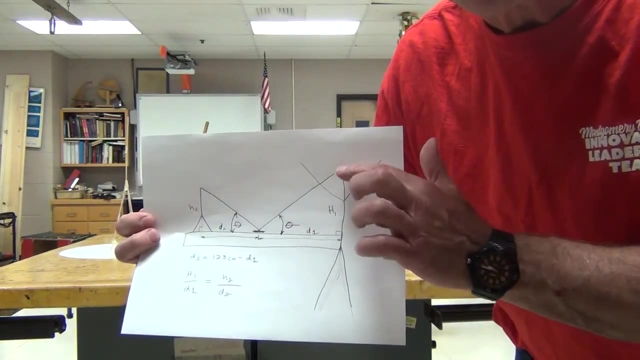 versus the other distance. I can calculate that other height right. It's a simple ratio, All right. so let's take a look at that Here. we have a beautiful diagram for your edification. Here's a particularly nice drawing of Mr Street looking down from the edge of the table to the mirror. 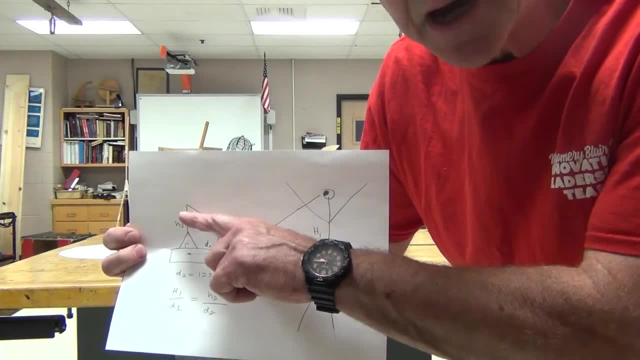 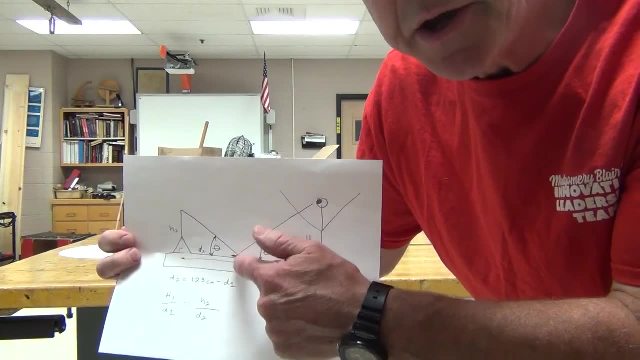 and then the line of sight from the mirror back up to the top of the tower, The distance I have here from the edge of the table to the center of the mirror. I know that distance because I can just read it off the meter stick. 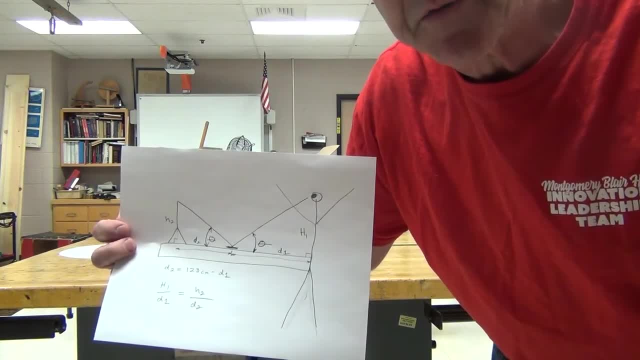 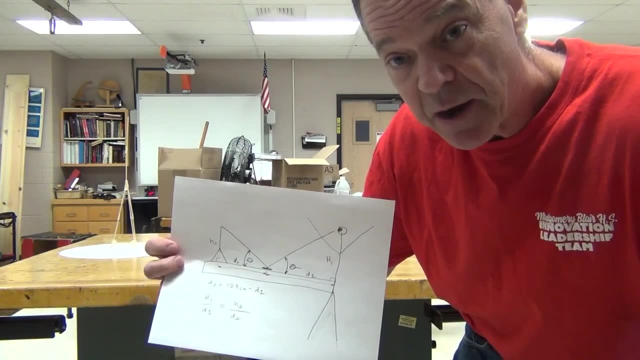 The other distance I can calculate by subtracting it from the known distance. I haven't moved my tower- The known distance from the edge of the table to the bottom of the tower, And then I can set up a ratio as you see there, where the height of the one triangle 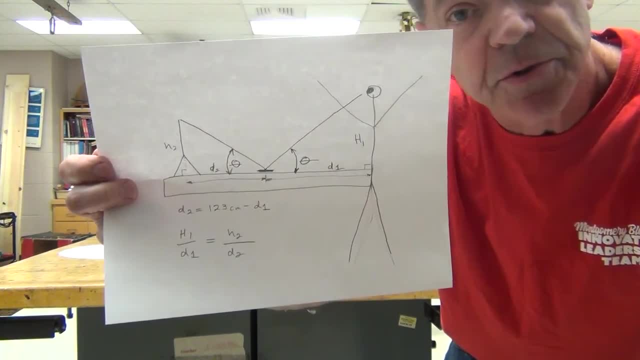 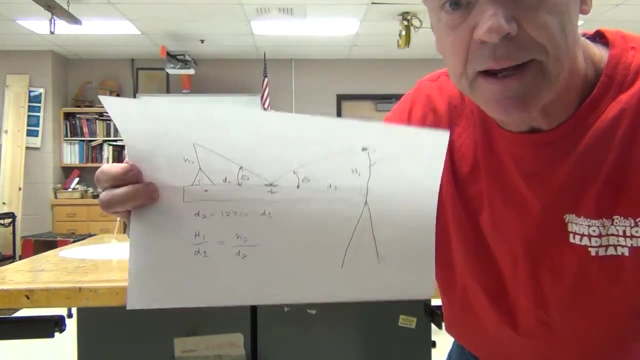 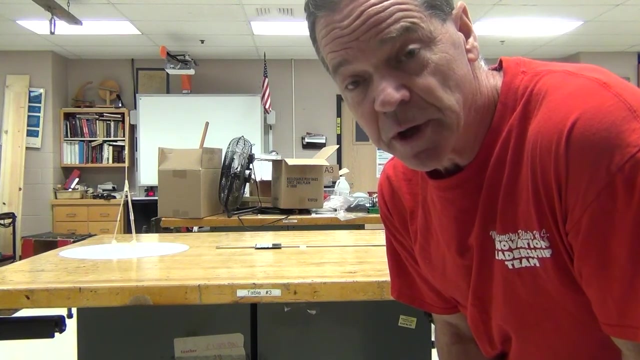 in relation to the distance is equal to the height of the tower in relation to the second distance. All right, pretty simple calculation. It helps a lot that the mirror has that aspect of those two angles being equivalent. Okay, so that's the way you do the mirror method. 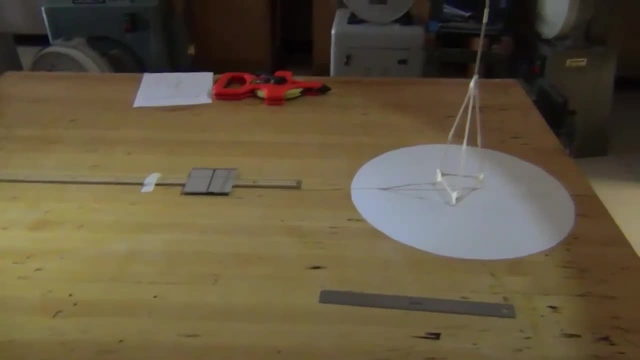 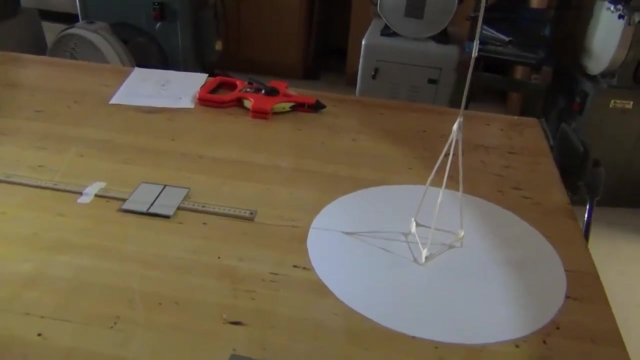 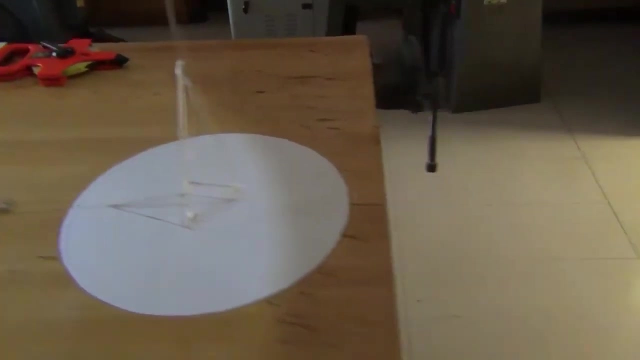 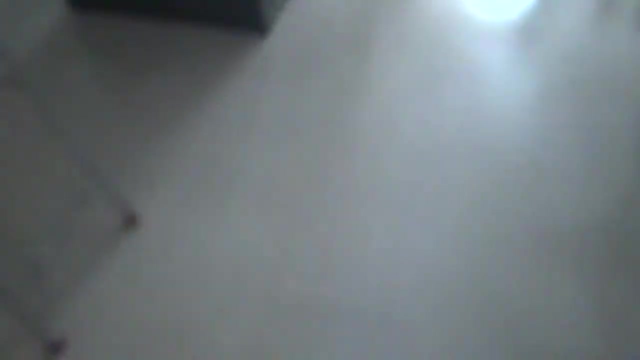 All right, here is the last measurement system, And this one also depends on similar triangles. What I have here is a light setup. Hold on one second. I'm going to kill this other light, maybe make it a little more obvious. Sorry. 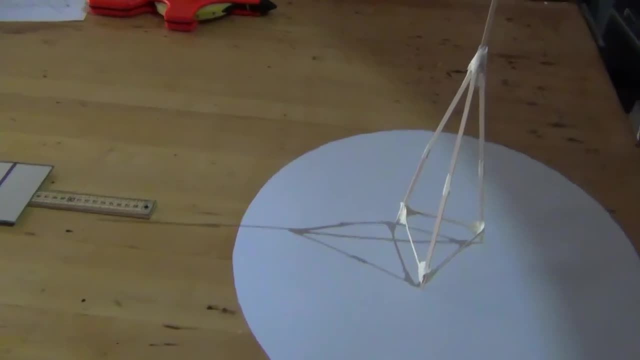 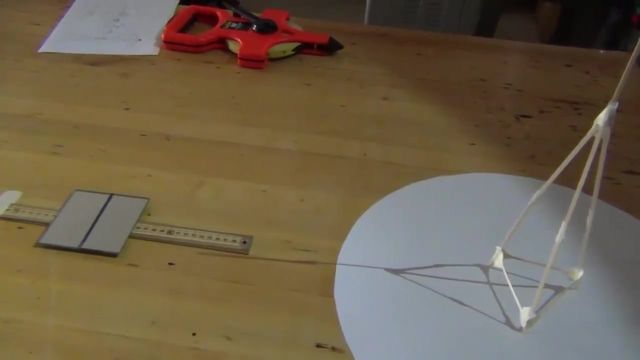 Okay Now, if we could go outside and use the sun, that'd be better, And we might try to do that. The good thing about my setup right at this moment is that I know this distance already. That tower is still sitting in the same spot. 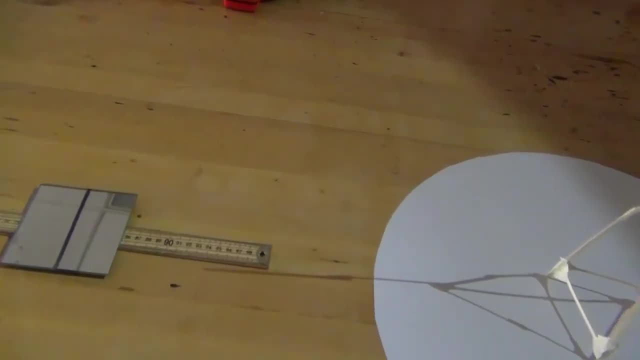 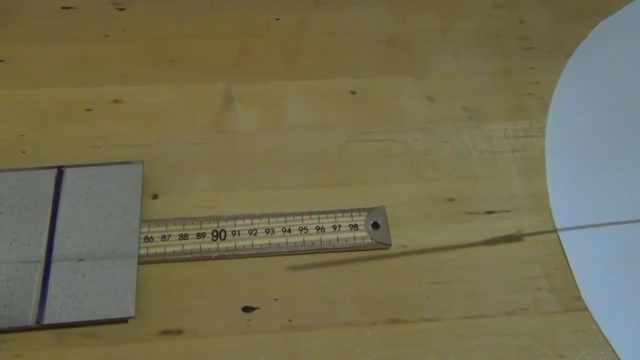 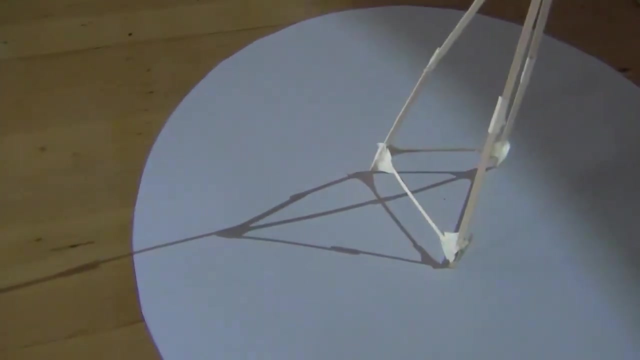 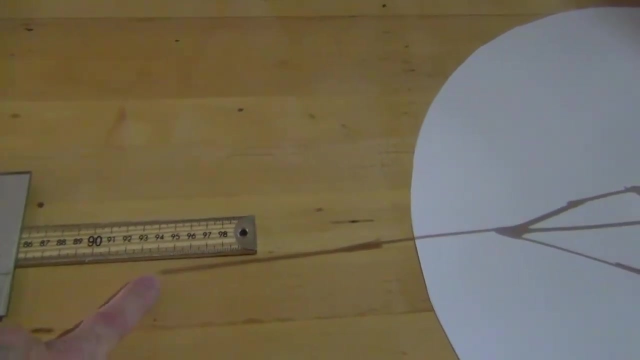 I still know the distance from the edge of the table. If I look really carefully right there I can see how that shadow lines up with the ruler. So I should be able to judge the length of the shadow based on knowing how far it is from the center of the base of the tower out to this mark right here. 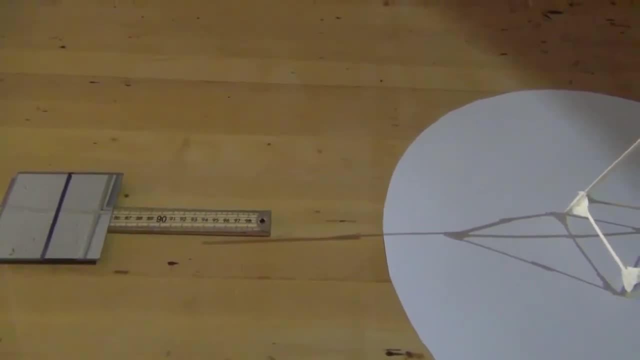 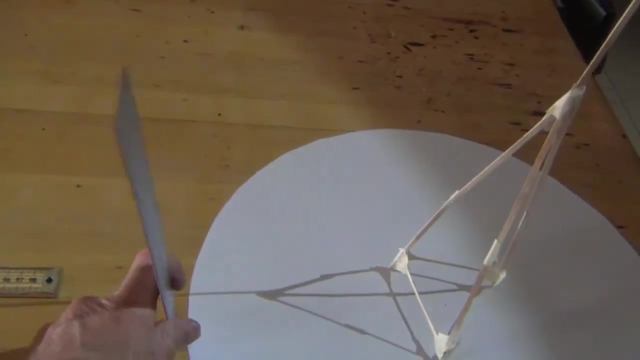 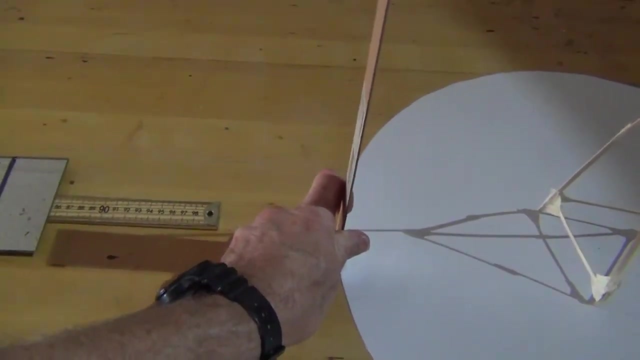 Right, That's good. So we can know the length of the shadow. We can know the length of the shadow of the tower, And this isn't perfect. But if we take a known object, an object of a known height, and measure the length of its shadow, right there, right. 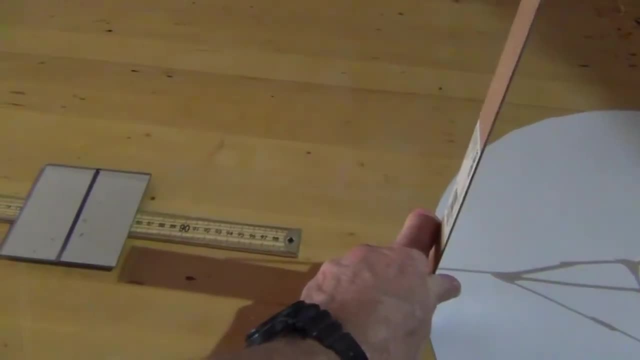 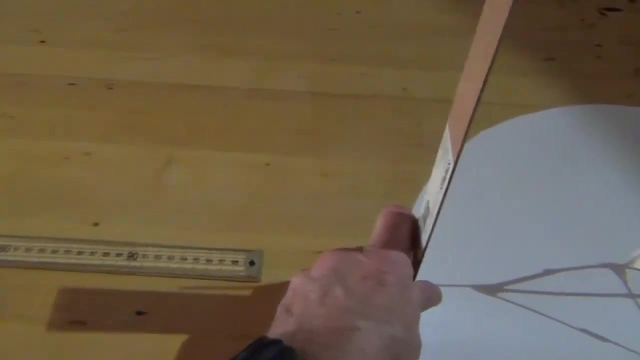 Well, we can figure it out easy enough: The length of the shadow there. right, I didn't take away the mirror, Hold on, Make this a little better without the mirror. We do like that. We can see right there where that shadow falls. 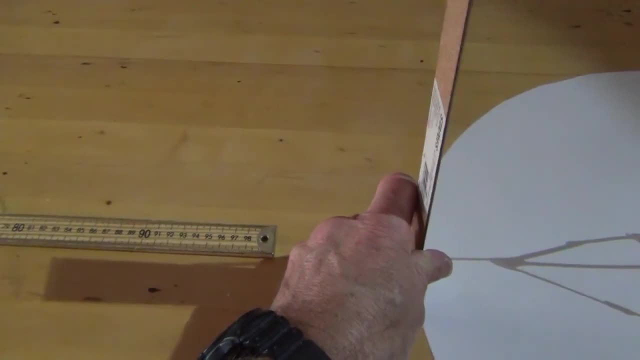 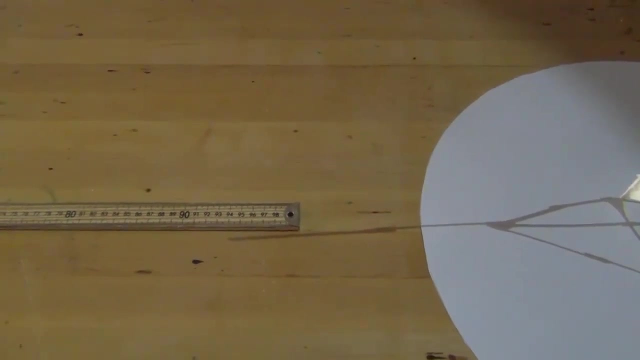 Get a length of that shadow And we should be able to come close based on similar triangles. Right, I'm going to try. if the sun will cooperate, I'm going to try to do an example of this shadow method, the real shadow method, outside with the sun. 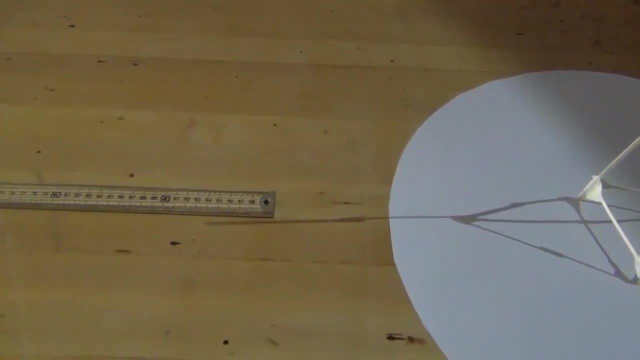 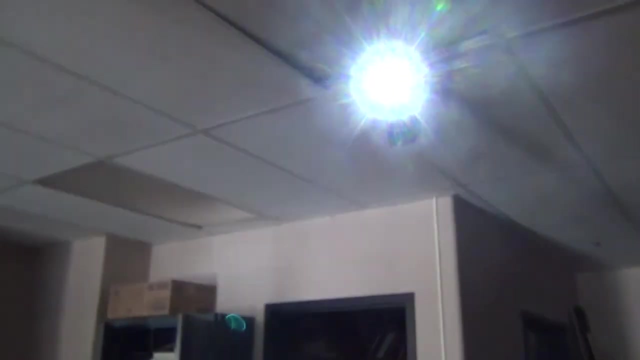 But for the time being, this will show you how you can do it. You have a nice bright flashlight like that one Right And a dark room. It doesn't have to be totally dark, Darkened room is good enough- And you can then set that light up. 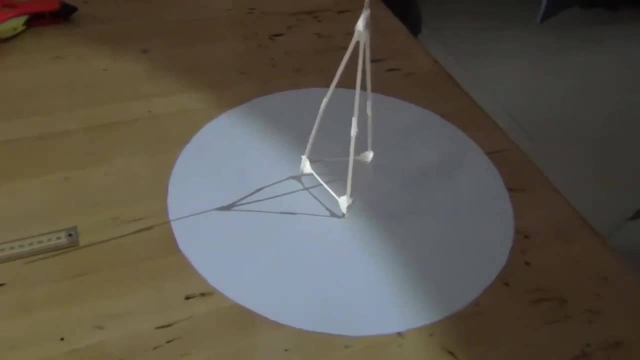 So it is outside the zone of exclusion, But it can shine a light through that zone. It's clear, And we can get a length of this shadow And do the same thing with this other known length. This is actually not a foot-long ruler. 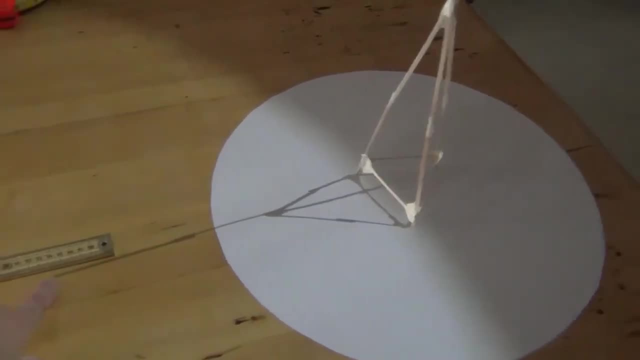 I mean, it's ostensibly a foot, But there's a little tiny bit on each end Longer than a foot, So you would need to take that into your, you know, figure out exactly how long the piece of metal is, Even though this is not a foot-long ruler. 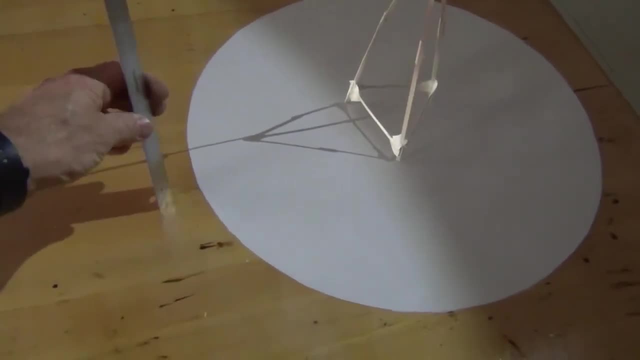 I mean, it's ostensibly a foot, But there's a little tiny bit on each end Longer than a foot, So you would need to take that into your, you know, figure out exactly how long the piece of metal is, Even though this is not a foot-long ruler. 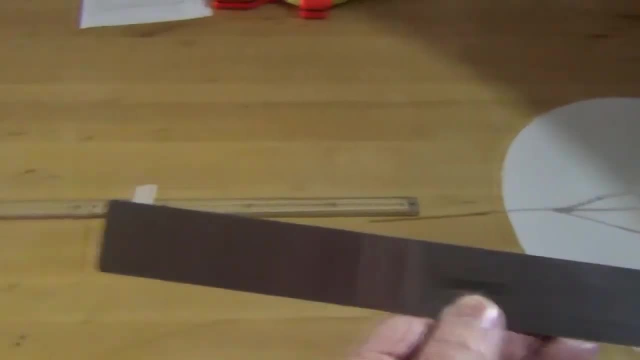 I mean, it's ostensibly a foot, But there's a little tiny bit on each end Longer than a foot, So you would need to take that into your, you know, figure out exactly how long the piece of metal is, Even though this is not a foot-long ruler. 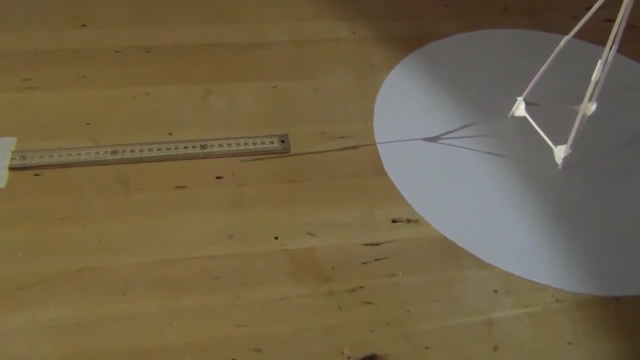 I mean, it's ostensibly a foot, But there's a little tiny bit on each end Longer than a foot, So you would need to take that into your, you know, figure out exactly how long the piece of metal is, Even though this is not a foot-long ruler. 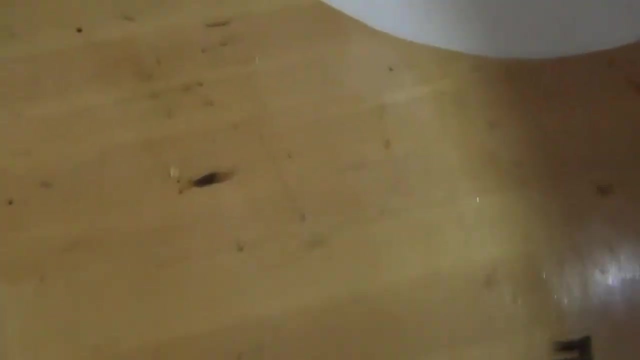 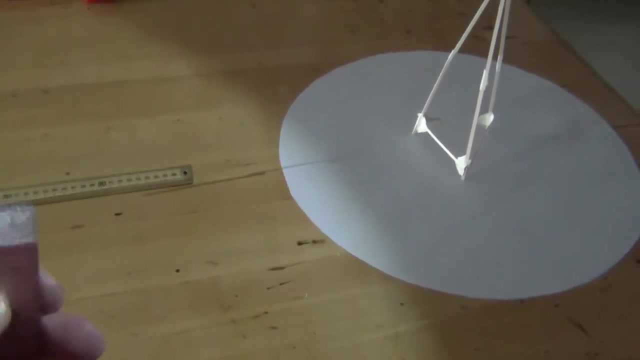 I mean it's ostensibly a foot, But there's a little tiny bit on each end. Longer than a foot. three-sixteenths of an inch or so, maybe an eighth, a little less than an eighth of an inch actually. 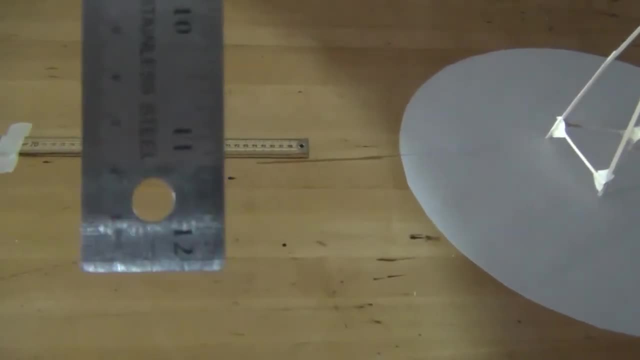 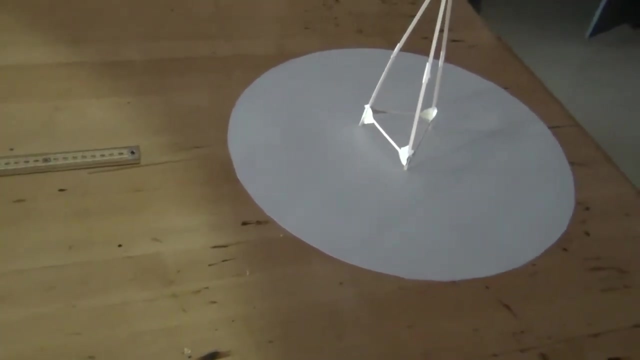 then the metal's a little tiny bit longer than the graduations. You should figure that out as part of your calculation. Do a ratio. you know the height of the shadow? I'm sorry. the height of the object is to the length of the shadow. 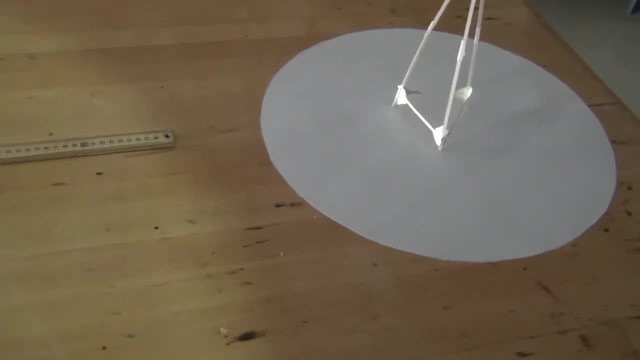 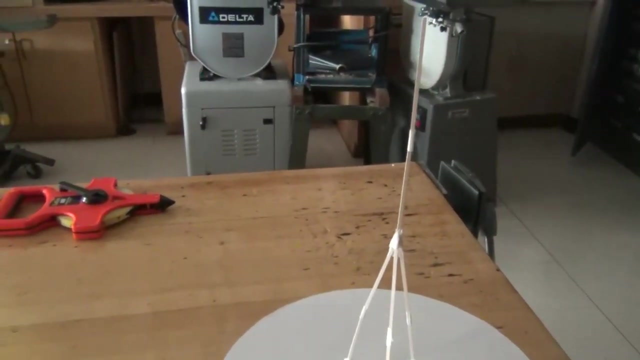 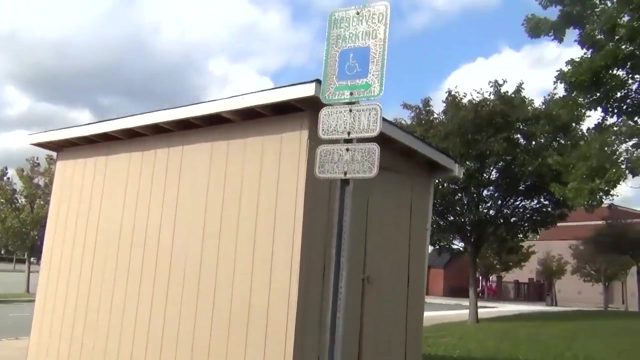 in the same way. in both it sets up similar triangles. Okay, and if I can, if the sun will cooperate, I'll go out and do a measurement there with some other things, see how well that works. All right, so here I am, outside of the school and I have found a nice pole sticking up here. 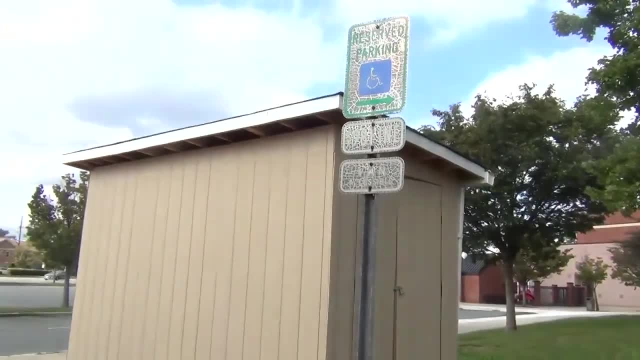 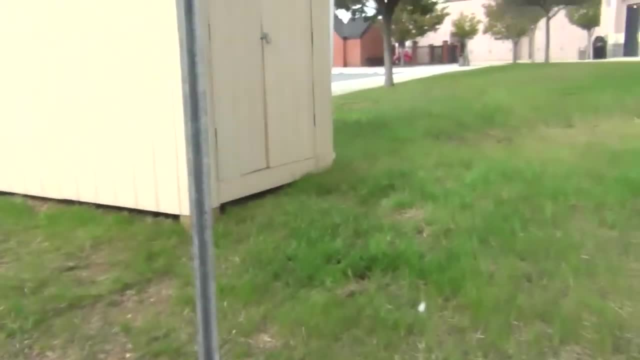 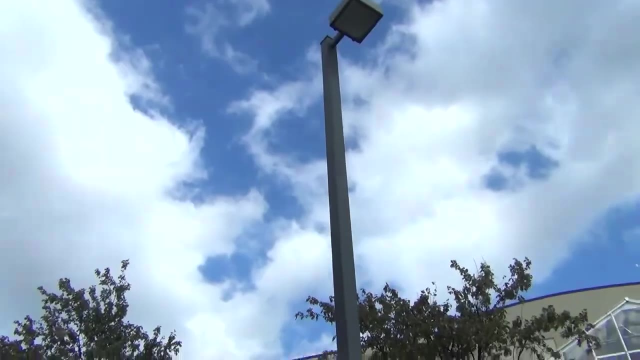 a no-park reserve parking sign. Of course it's a little useless right now, since they parked the portables right here in the spot, but okay Anyhow. then we've got a lamppost a bit taller and the sun keeps playing hide-and-seek with the clouds. 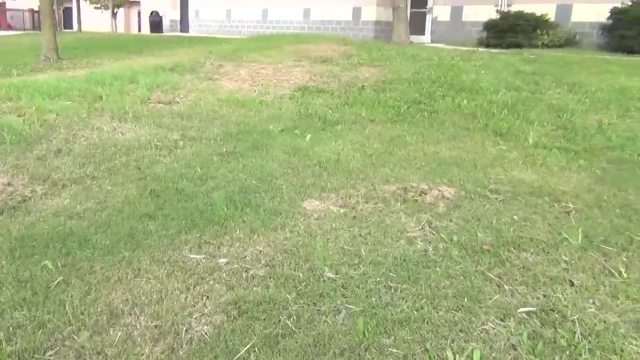 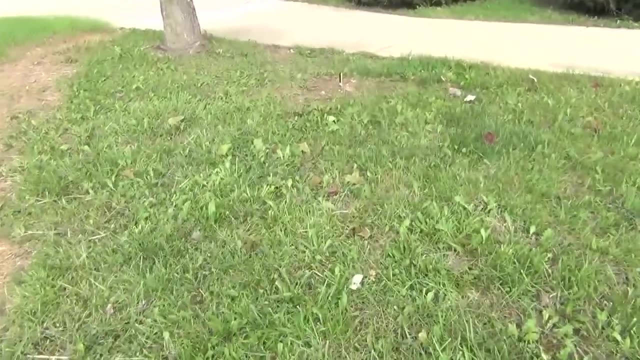 but what I did was when I came out, when the sun was bright, and I stuck a screwdriver in the ground at the end of each shadow. so the end of the shadow for the lamppost is right here, right about there. 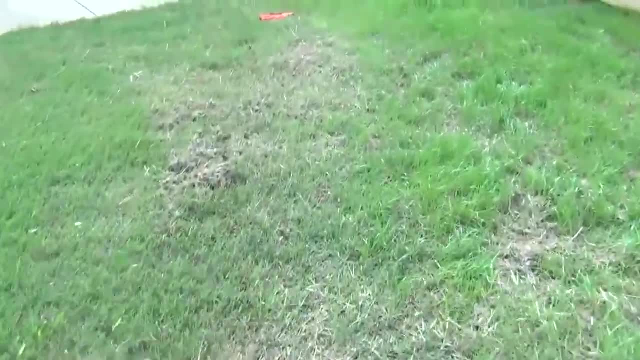 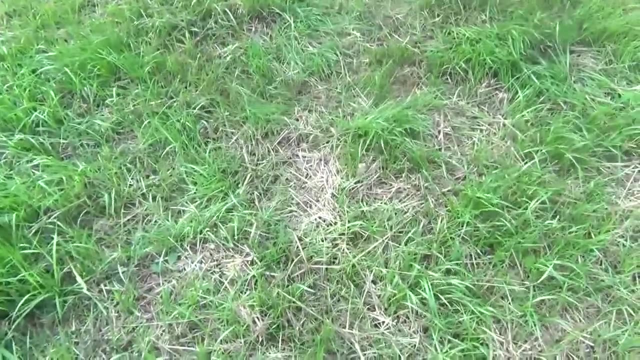 and the end of the shadow for the lamppost is right here, and the end of the shadow for the signpost is hiding in the grass here somewhere. Where did it go? There it is. There's the end of the shadow for the signpost. 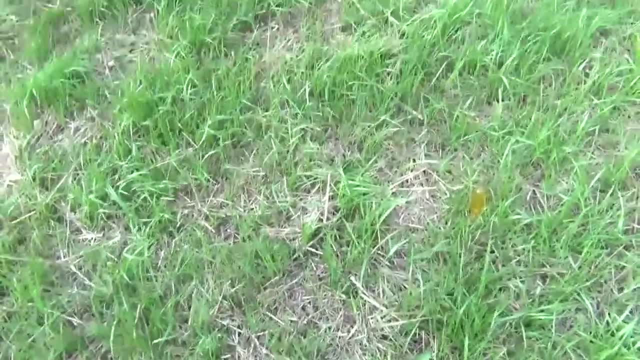 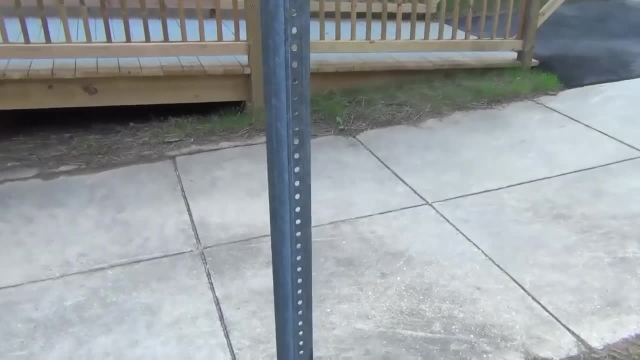 So now that the sun's going to hide behind the clouds, the shadow's not so obvious anymore. Maybe it'll come back out in a second, we can see it again, But I'm going to go ahead and measure the height of this lamppost. 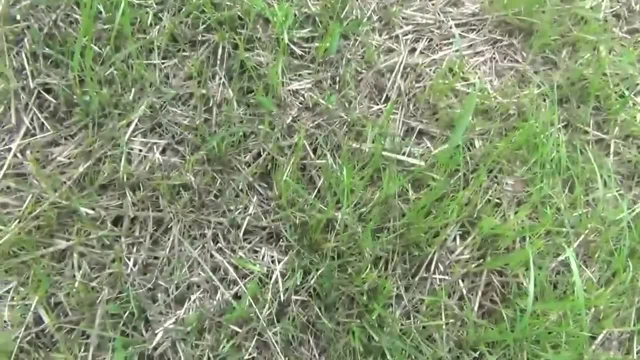 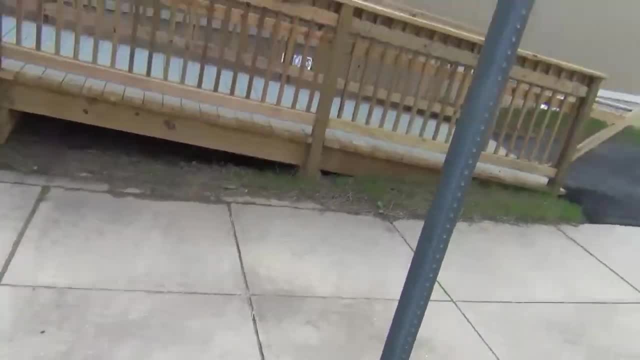 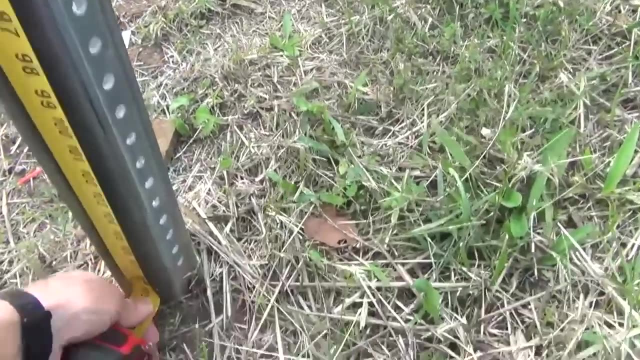 and let's see if I can do this one-handed. I might be able to get it. Oh yeah, look at that. Okay, so that's hooked on the top of the lamppost. I'm going to go down here to the bottom. 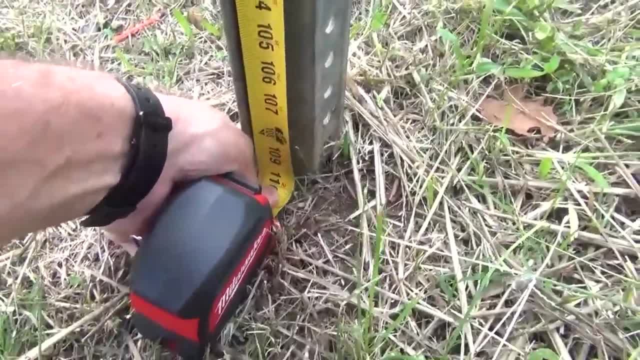 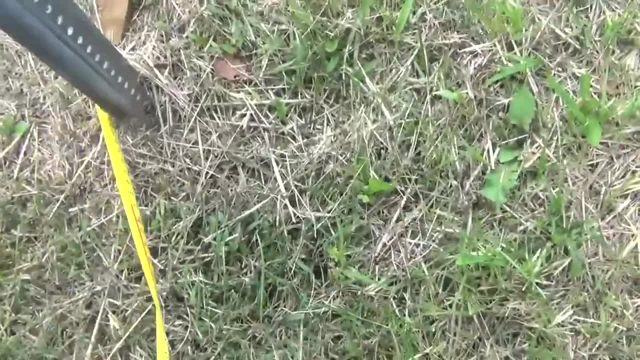 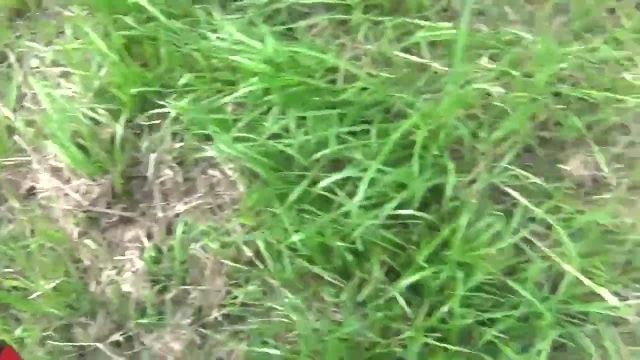 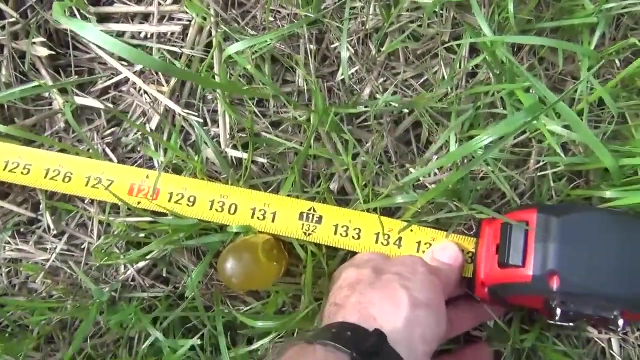 This says it's about right, about 110 inches. Okay, 110 inches for the height of the lamppost, and then we'll hook it on here and we should get okay. it says 131 inches for the length of the shadow. 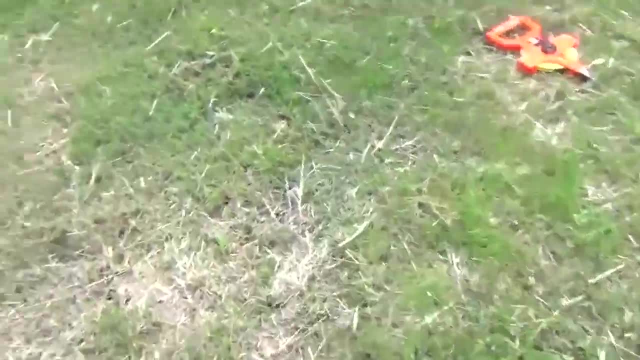 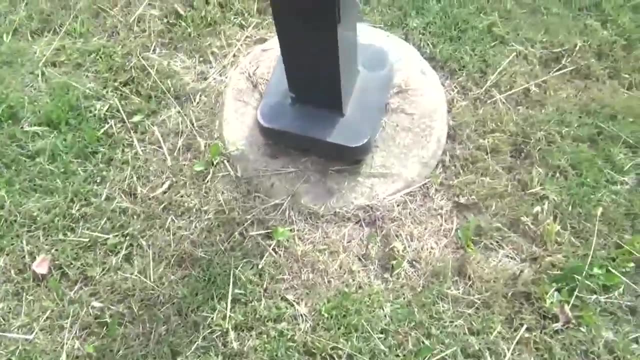 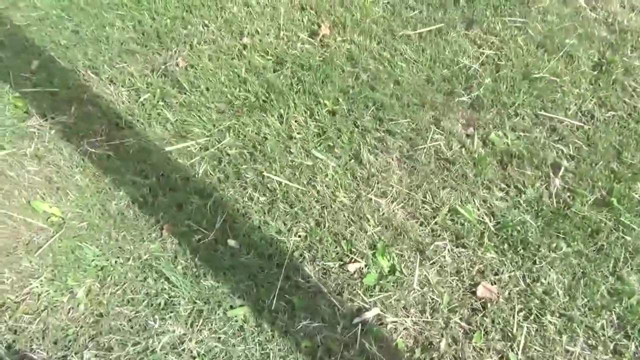 So 110 to 131, and the length of this shadow. let's see if we can get it. Okay, Oh, I may need this. Okay, I'll probably need the other measuring tape, don't I? Yeah, I will. 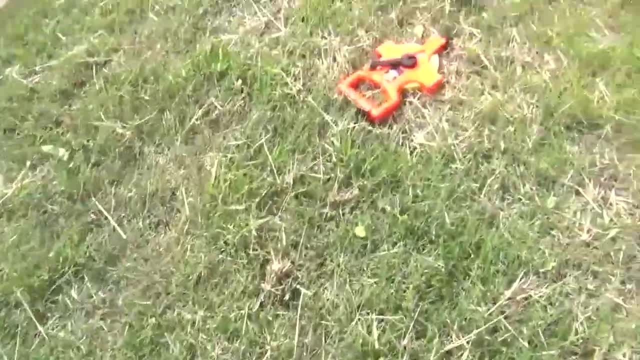 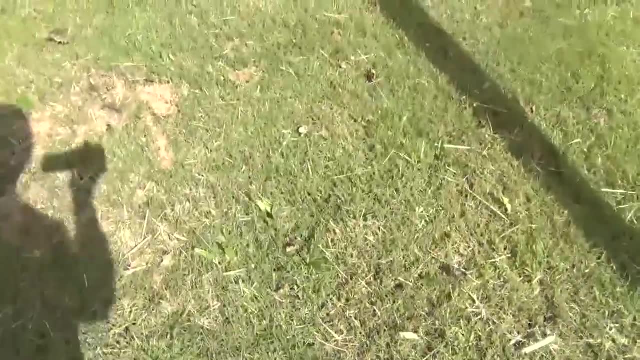 Let me get the other measuring tape. I have a longer measuring tape because I'm pretty sure that other one won't be quite enough. Oh, look at that Boy, look at that beautiful shadow, Isn't that great? There you go, the sun came out. 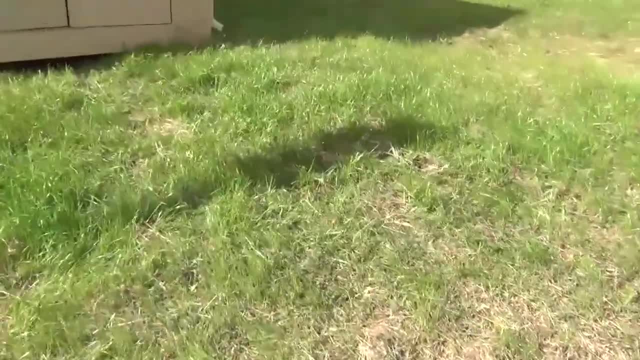 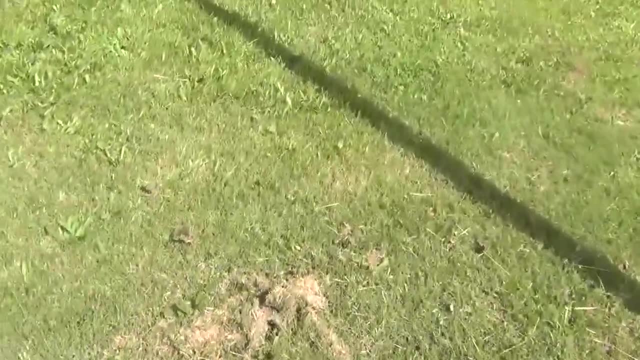 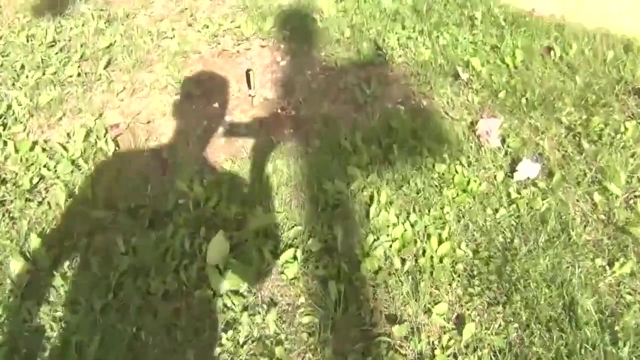 There's the shadow there, And there is the shadow there. Okay, you can really see them stand out against the grass right now, can't you? That's just great. Okay, Let me. uh, I'm just testing out here to make sure I've got the right. 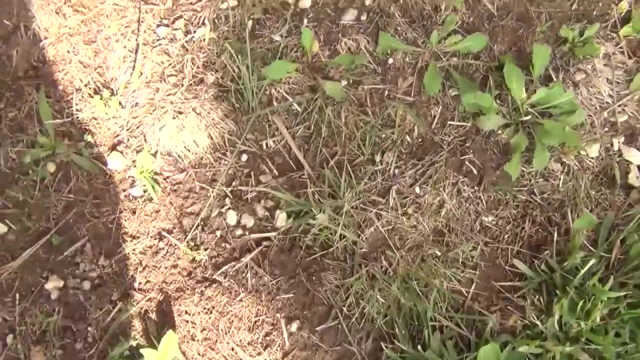 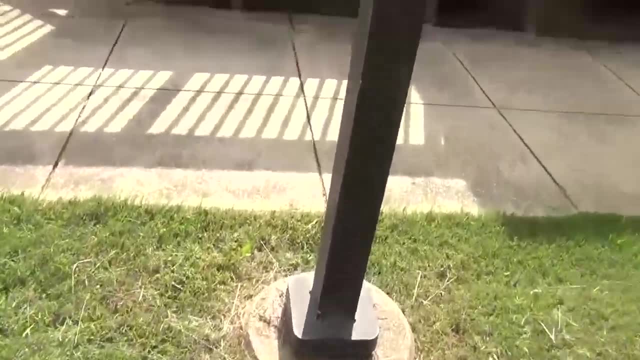 the right end of the shadow. This should be it right there. Okay, Hopefully we didn't mess it up by by moving it. Okay, So I'll go over here and hook, hook the tape on this guy. See if it'll stay there. 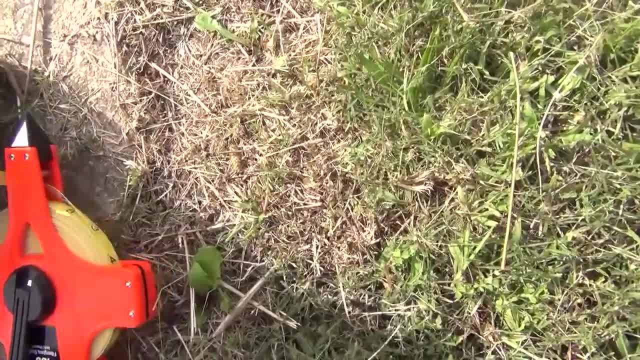 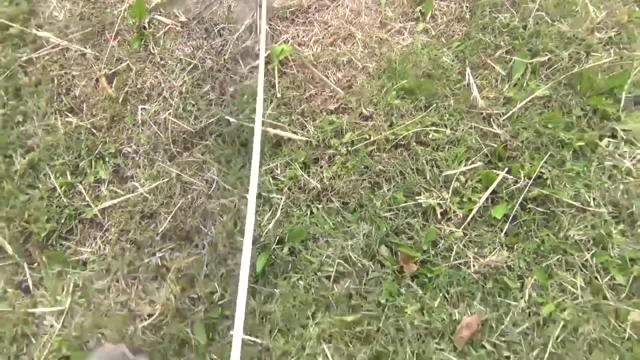 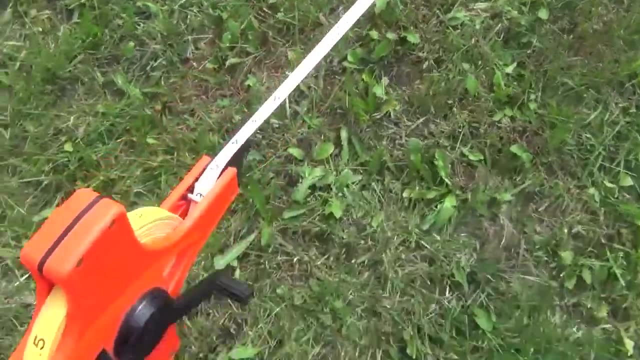 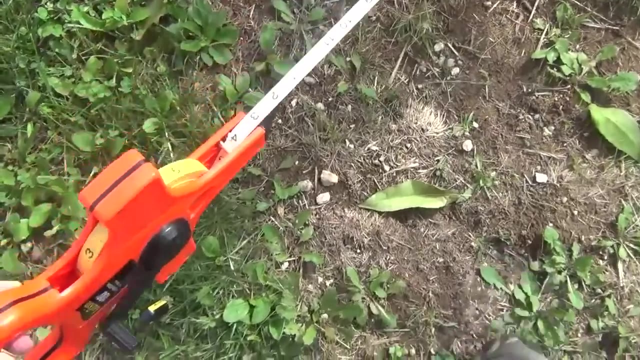 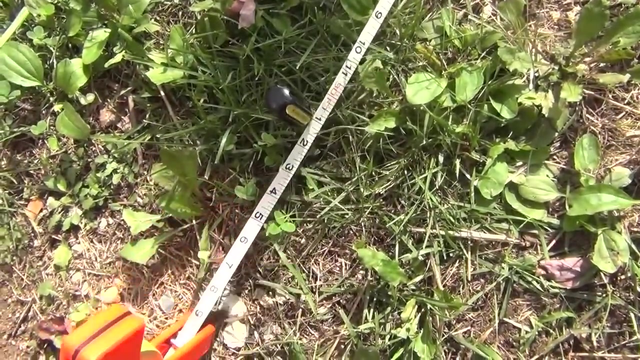 Maybe on this side if I'm lucky. I'm sorry, I've almost got it, So you can see. Checking out the tape: Okay, That says 30.5.. 3.1 feet Or, uh, actually 30.. 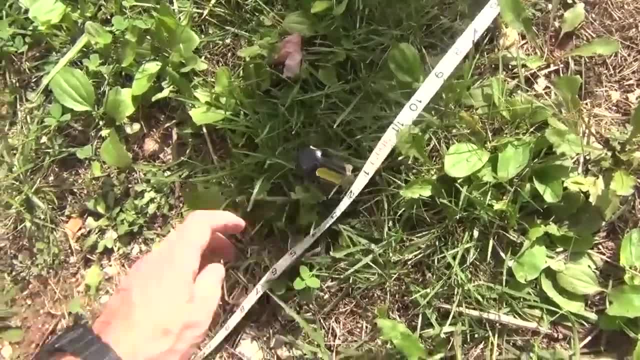 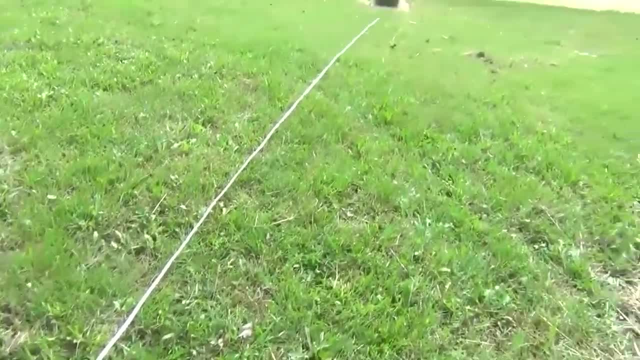 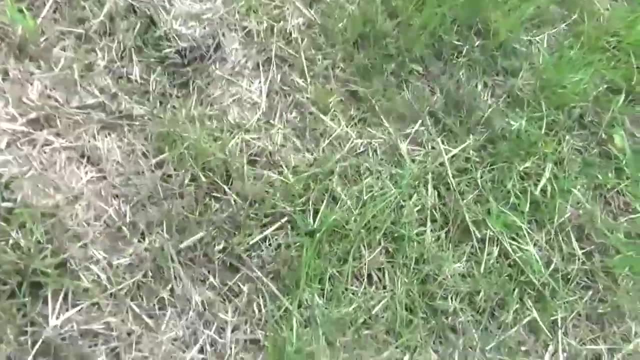 That looks like 30 feet one inch, 30 feet one inch, Okay. And the other one was 110 to uh, 100, shoot 13.. Right, 110 to 113 inches. Did not move that screwdriver. 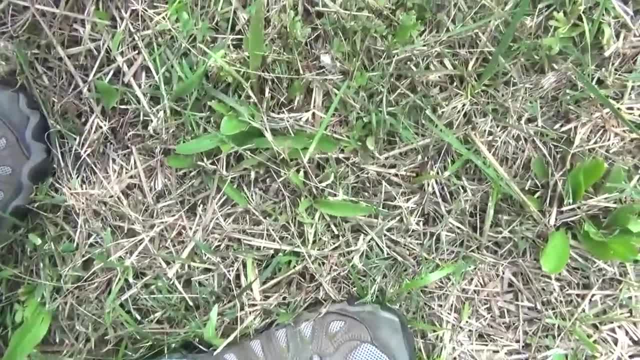 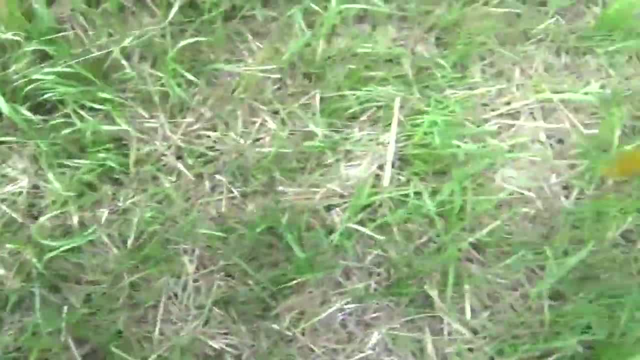 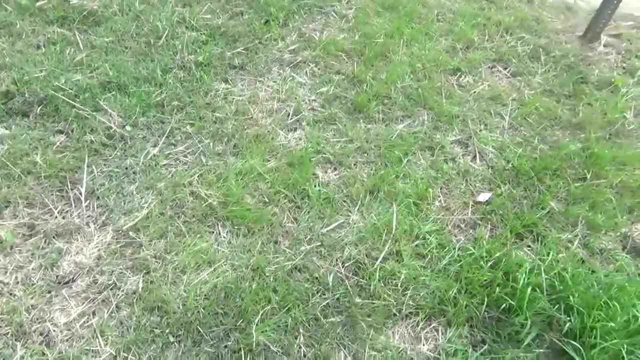 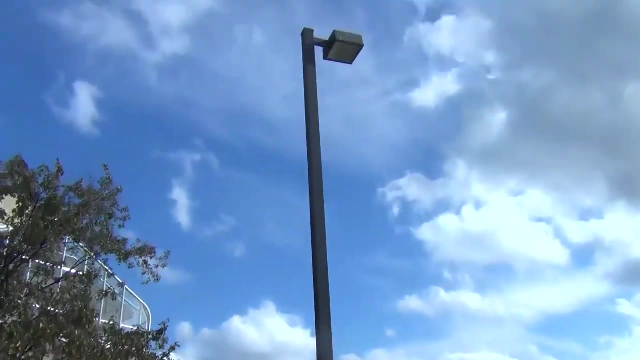 Double check that, Okay. Okay, Oh, I'm sorry. 131.. 110 to 131.. Okay, That's great, Then we'll- uh, I'm gonna leave the calculations to you. You tell me how tall that lamppost is, to the very top.